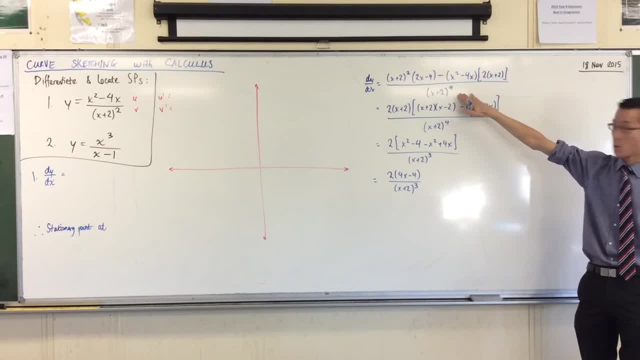 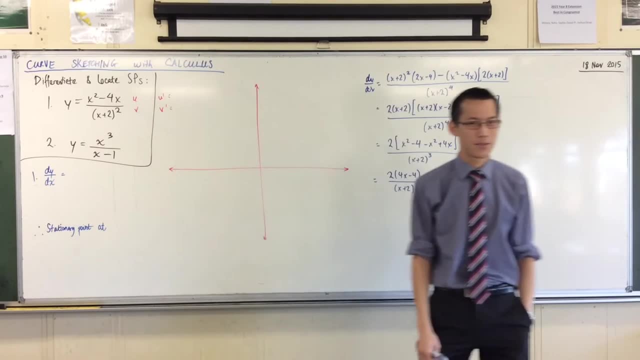 There's my numerator and there's my denominator. Now, the denominator is gross, but that's okay. I'm only trying to find stationary points, right? So the numerator is really the part that matters for that, okay, When I get to this point here. okay, can you see what I've done? 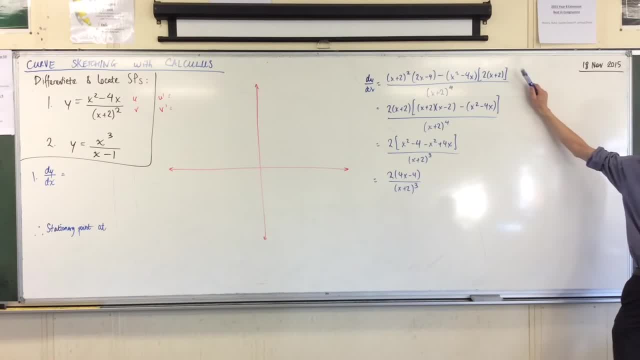 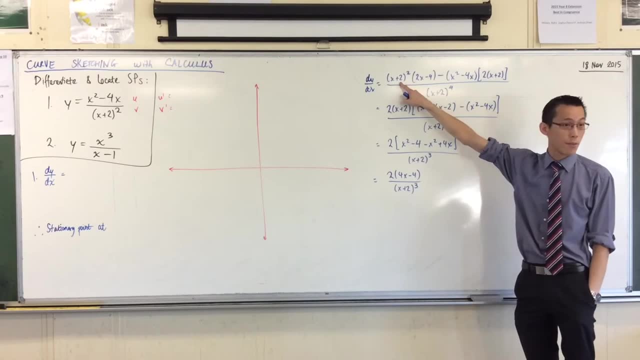 I'm trying to be smart about this. I could have just expanded the lot here like it's doable. It's just not very efficient. okay, You see, from here, if I expand it from there, I'm going to get three terms out of that, and then you go three times two. 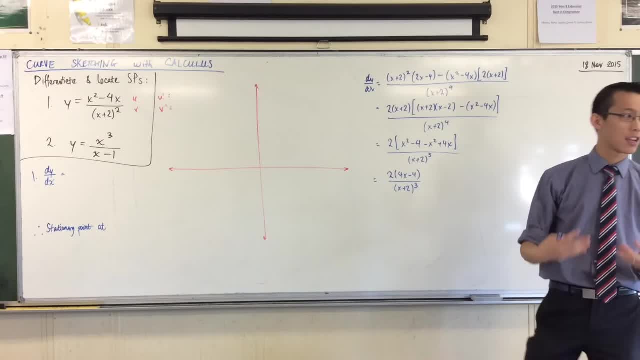 there's six terms already. Just the number of places where silly errors can creep in. you're just hurting yourself, right. So to be smart about it, I look at this and I say: wait a second, I have some well, and I ought to expect this. I have common factors happening up here, right? 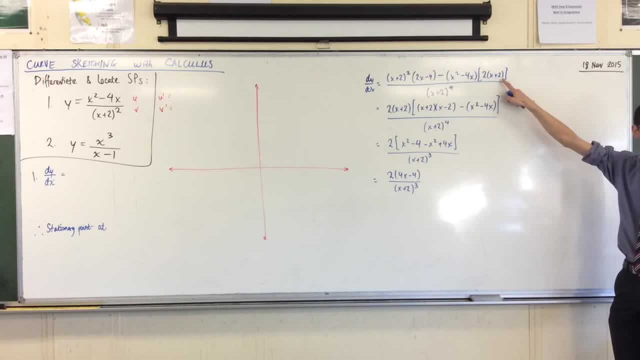 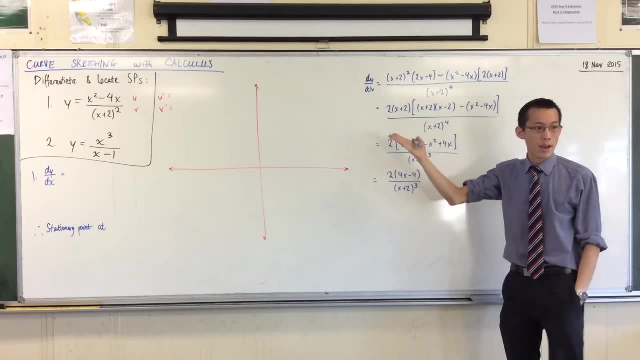 There's an x plus two here and an x plus two here. yeah, There's a two here, and this is also something which I can factor as two out of. So that's how I pull two times x plus two out the front, okay. 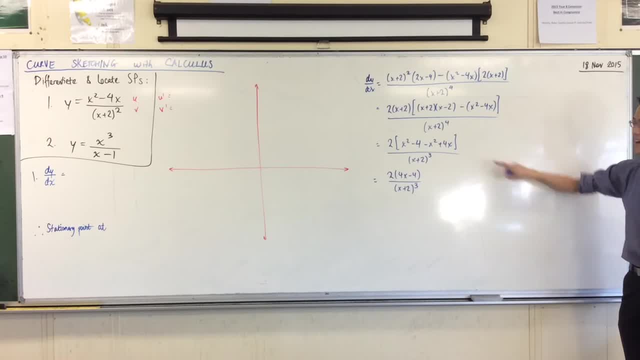 And this is what I'm left with Now, from this line to this line. I'm a bit naughty. There's something I haven't written here. What have I done? I've done two things, from line two to line three. What are the two things? 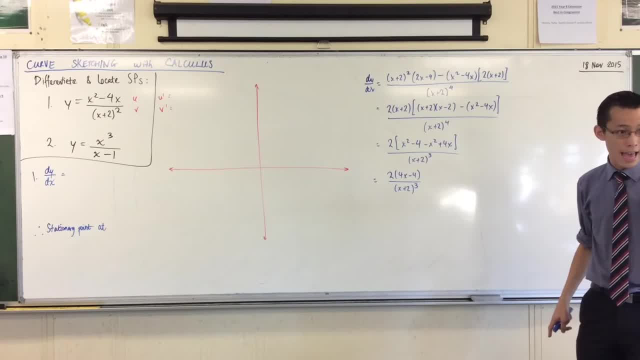 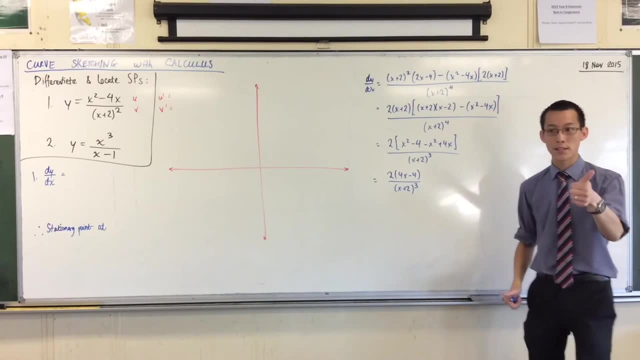 x plus minus two U. Okay, number one. I've done difference of squares there, so that's good. You know, rather than getting many, many terms here, I've just got two. That's good. That's the first thing. 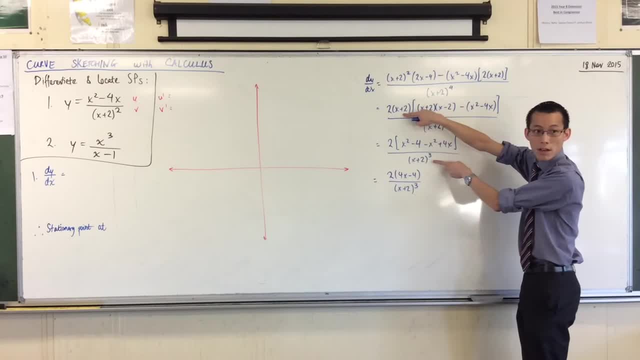 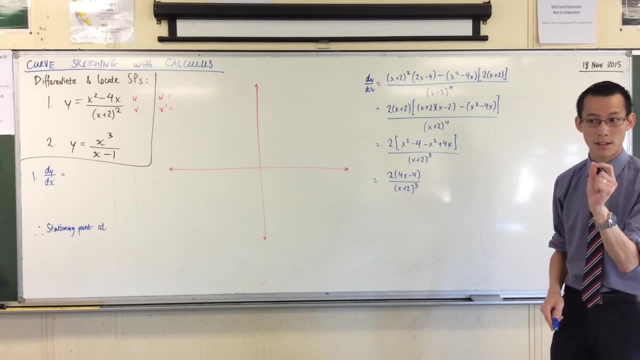 And the second thing I've done is I've cancelled out the x plus two down here. That's why I only end up with three of them, not two. But you can't just do that right, You can't just cancel things out. You can only do that in certain cases. 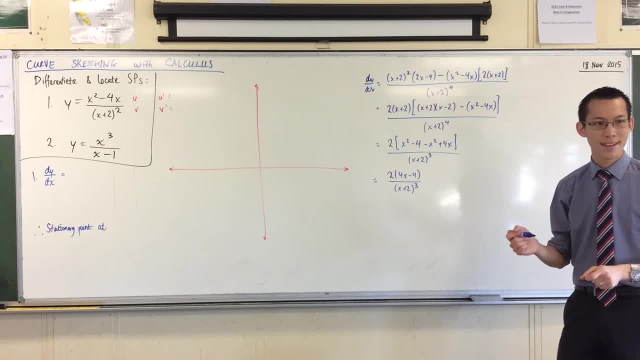 Why can't I cancel x plus two? Because it's a square at the bottom, so it can. you know X is. you already know x is not equal to two. Now, okay, there's a. There's a couple of reasons. 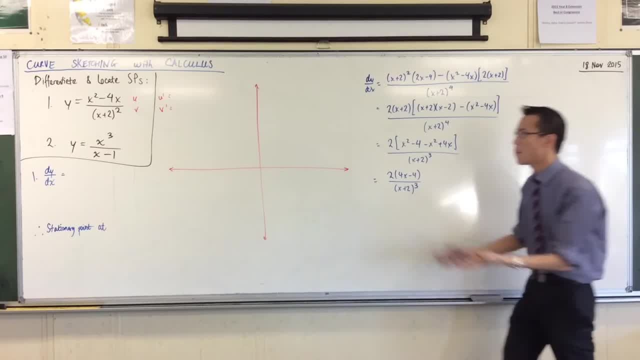 Well, Brendan, do you want to add? Yeah, okay, Um, the first thing is, remember, I am graphing right, So you come back to this guy Now, even though I haven't gone through this process yet. 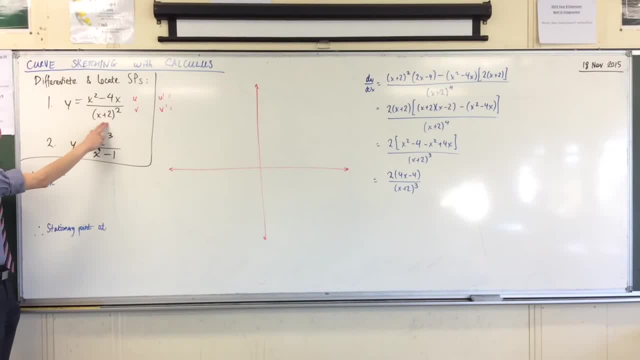 because I'm going to be curve-sketching. you know that this is going to have an asymptote. right? This guy has a discontinuity at x equals negative two. right. So he doesn't exist there. So if he doesn't exist, I don't care about that point. for the first derivative either. 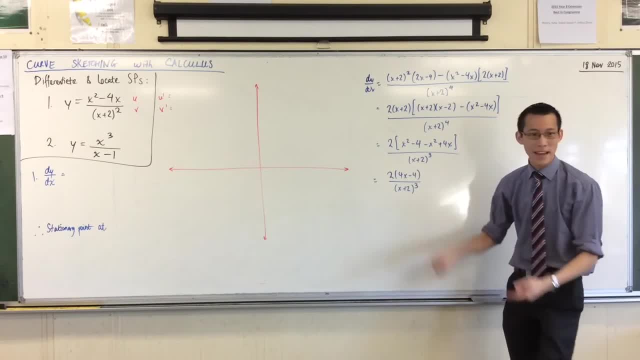 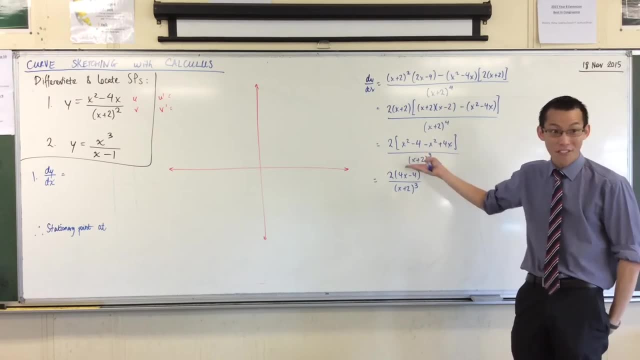 That's the first point. Secondly, because on the denominator I still actually have an x plus two. right I have an x plus two term. Um, I haven't gotten rid of the discontinuity. The discontinuity is still right there on the denominator. 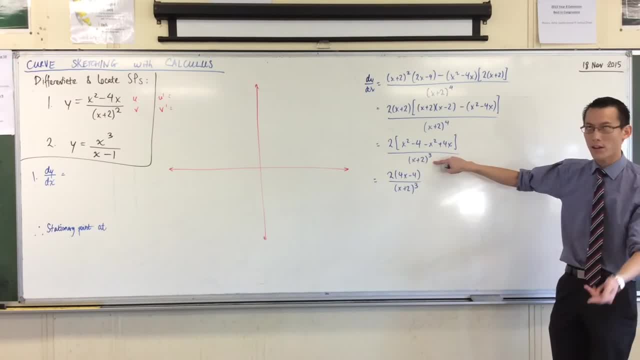 It's the same discontinuity with this as with x plus two squared or x plus two to the one or x plus two to the hundred. I have preserved that, But anyhow, I'm still going to say the reason why I can cancel. it is because 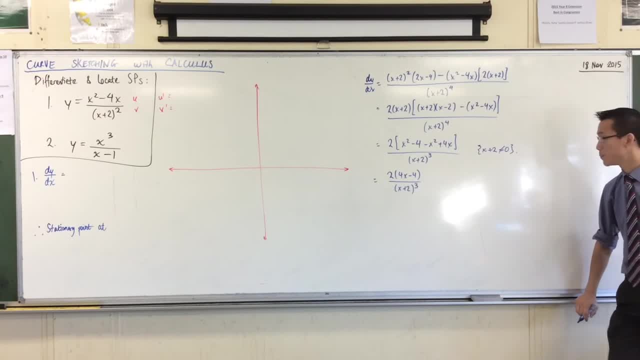 Sorry, uh, yeah, that's not going to be zero. X can't be negative two. okay, And you boil it down to here. okay, And this is my second last step before I can actually say what is the simplest form. 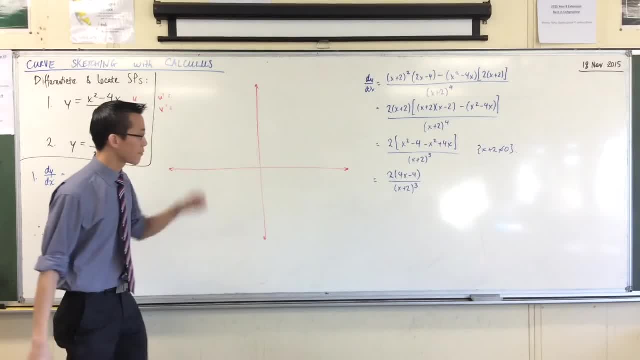 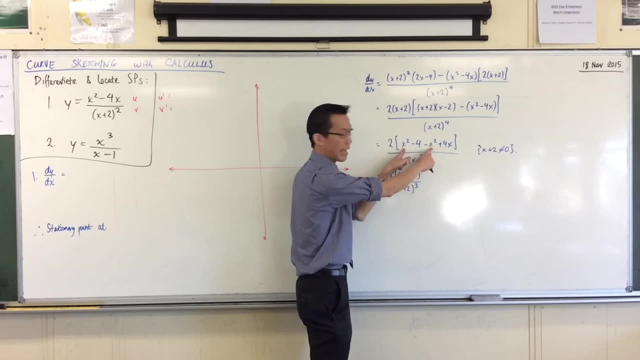 I can write the derivative in. Oh, I was just going to ask: why did you factor out the two and not eight? Yes, okay, just because I'm not finished yet. Oh, okay, Um, from this line to this line, all I did was I cancelled the x squared, which left me here. 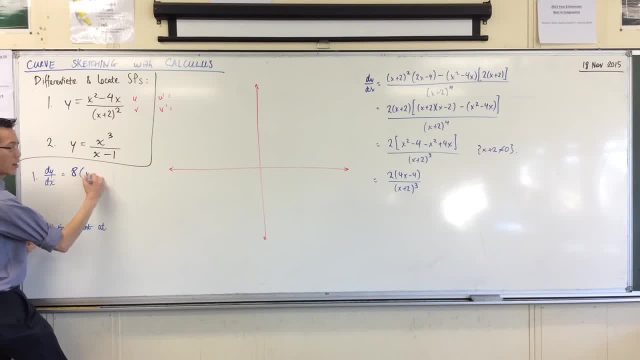 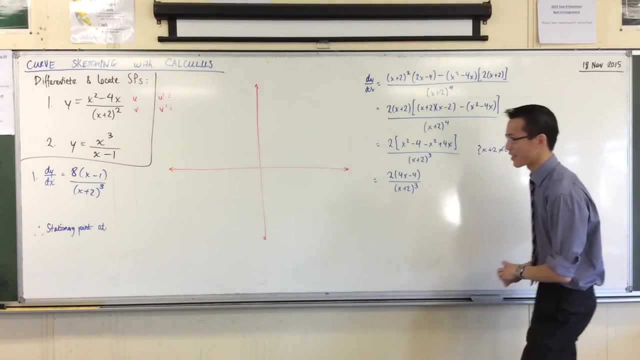 And now I'm like: okay, I'm ready to go. Here is my factorization x minus one, And it does tidy up quite nicely, okay. So what conclusion do I draw from this? Like, what was the point in me finding this derivative? 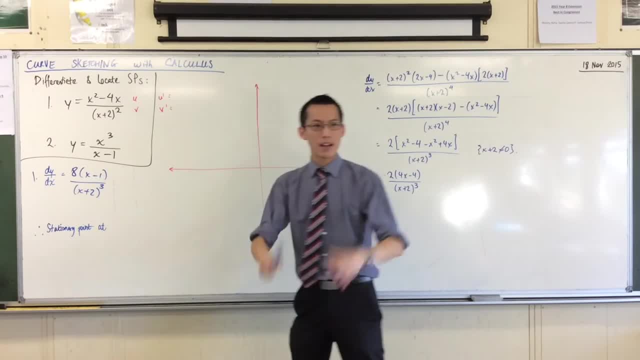 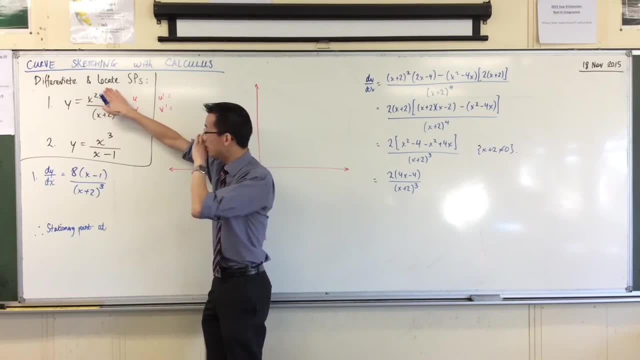 This: I want to find the stationary points. I want to find the stationary points. okay, Now just let me again get in your head the difference between- excuse me a question which says differentiate, find stationary points. that's the question, as opposed to. 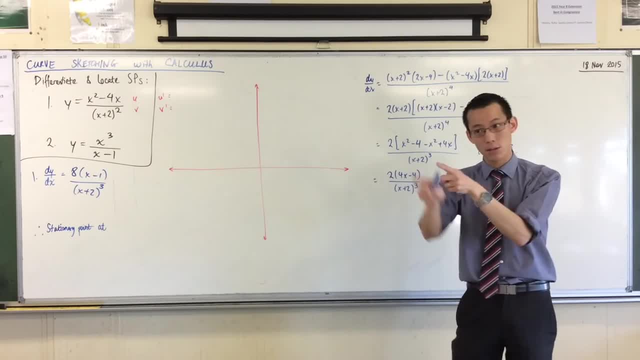 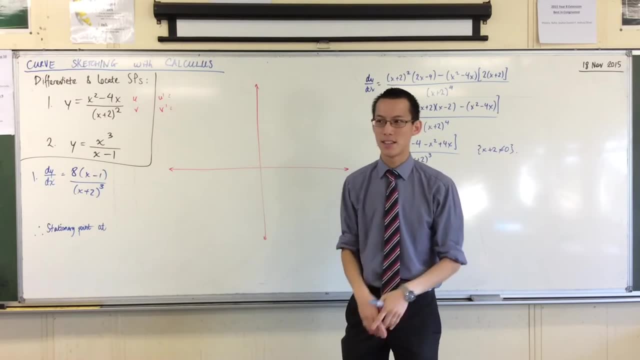 differentiate and find stationary points. that's not the question. I'm just using that as a means to an end. The real thing I want to do is curve sketching. So here I'm going to be a little more fast and loose with my interconnecting sentences. 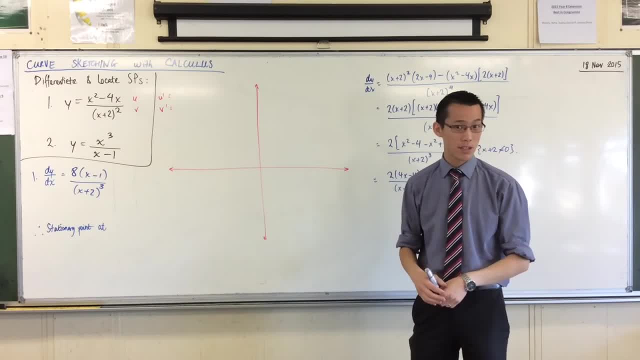 and justifying this that the other. I'm not going to determine the nature of the stationary point, Not only because I haven't been asked to, but because, when I start to put in the rest of the pieces of information that I know about this, 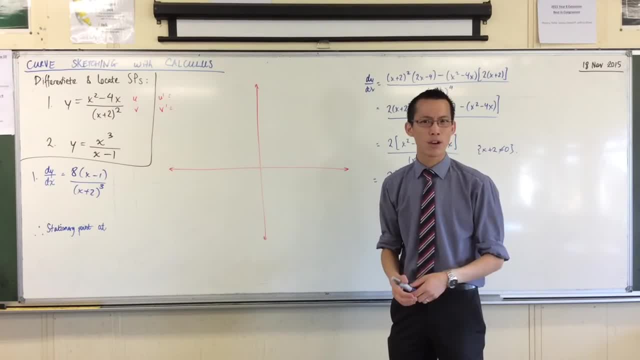 before calculus: you don't need to do that Like it's a bit overkill really. I would only do that if that was the actual question. Find the stationary points and determine their nature. okay, If the real question is curve sketching, draw me a picture. 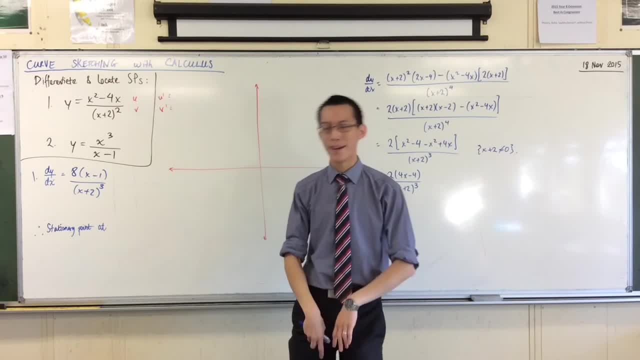 the nature will kind of emerge out of that and I don't need to do it formally. I don't need to draw up a table of values, I certainly don't need to go to the second derivative, which would be rather a pain in this case. okay, 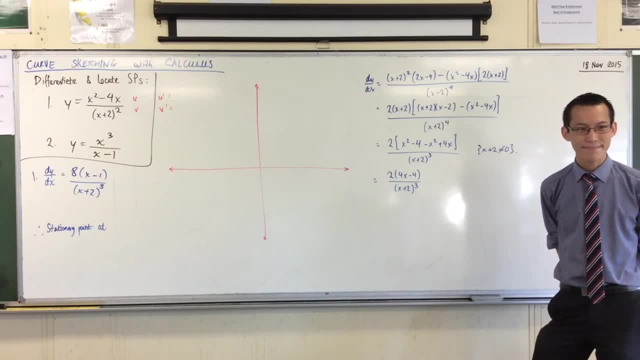 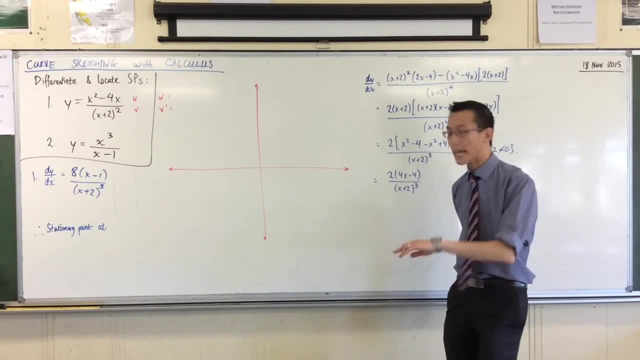 If the stationary point was like 0,, though, then you would have to test it. If the stationary point was like even x equals 0?, Because it might be a point of inflection. Okay now, like I said, interestingly enough, we will get to that when we go to this question. 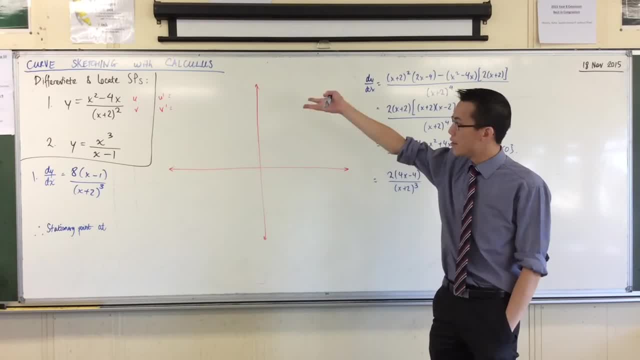 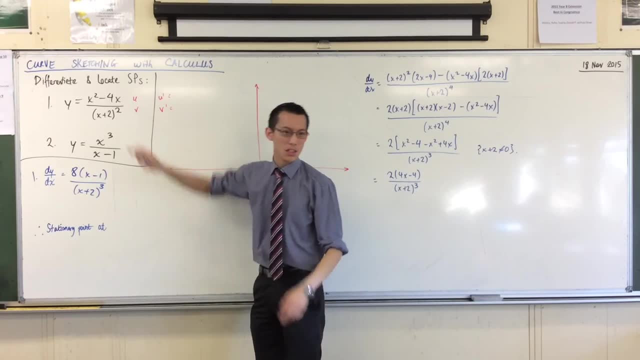 but we do not need to like we've done. these are called rational functions, right, Because it's a function which has a fraction in it, and that's what gives you these asymptotes and the weird behaviour and that kind of thing. 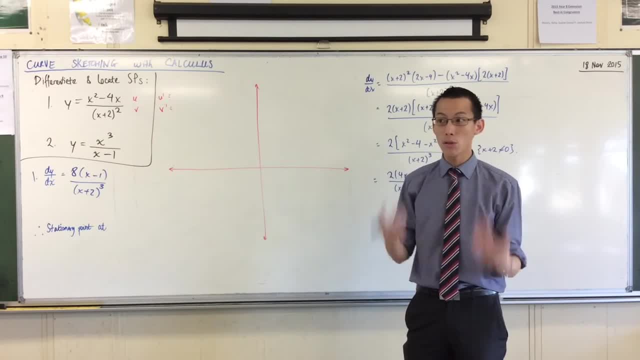 We have been looking at those way before. we learnt calculus And we knew lots of things about them. The main thing we were missing was: well it turns, Where does it turn exactly? And you had no tools to work out to calculate those positions. 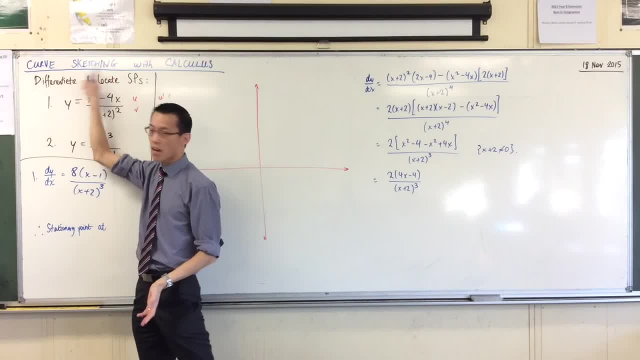 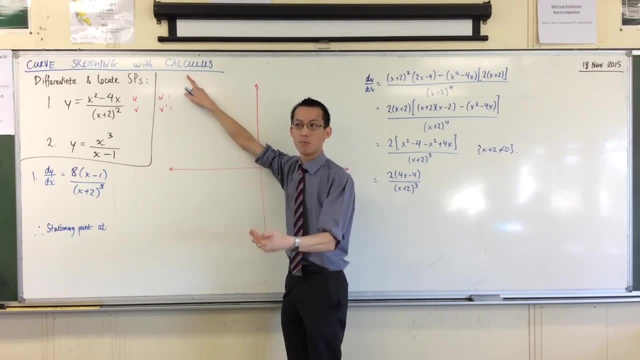 But now you do. Okay, so in some senses, the lion's share of what we're doing here you already know. you don't need derivatives, you don't need second derivatives. This just kind of adds on a little bit of precision. okay, as you'll see. 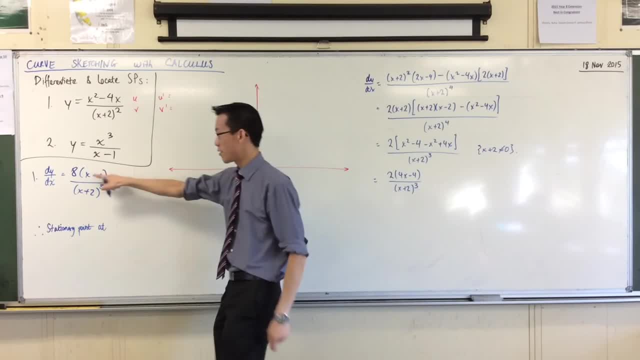 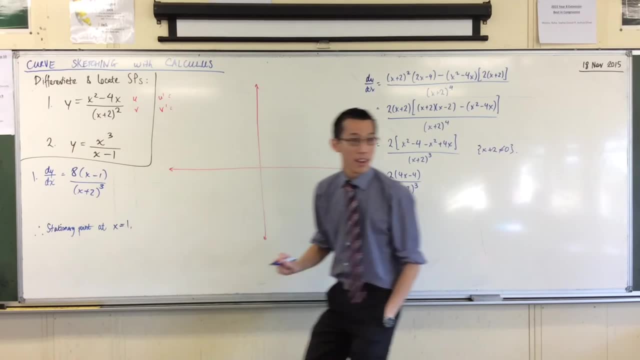 So where is my stationary point? You can just read it off, right, It's when the whole thing is 0, so it's x equals 1.. Okay, Sorry, say that again. Okay, yeah, good, So I've got my x coordinate. 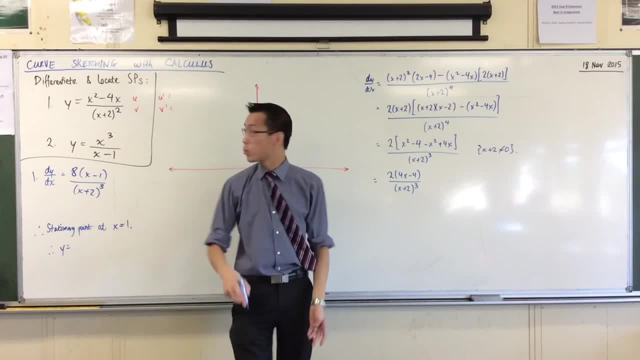 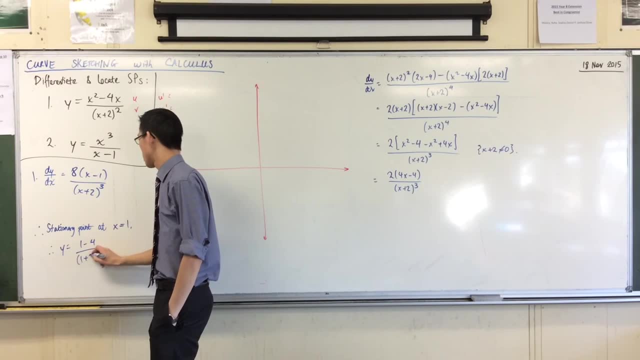 You're going to my next step. Therefore, for x equals 1, here's my actual function here. So I'm going to go 1, take away 4 on 1 plus 2 squared, Are you okay with that? Like I'm just straight substituting in: 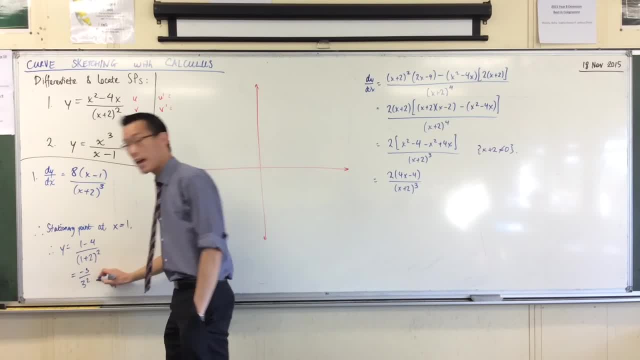 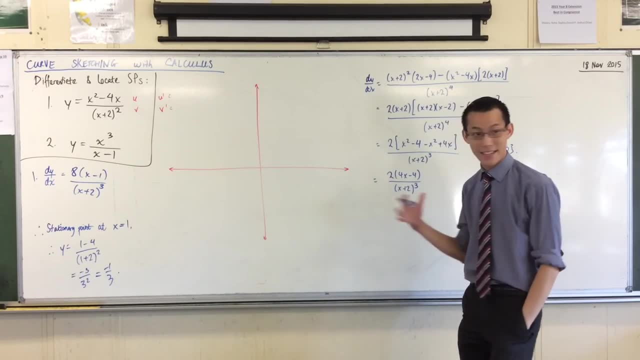 That looks to me like minus 3 on the 3 squared- which would be a bit naughty because I ran out of space- Minus a third. Are you okay with that? So now I have coordinates. Now I know when I start to get to the graphing. 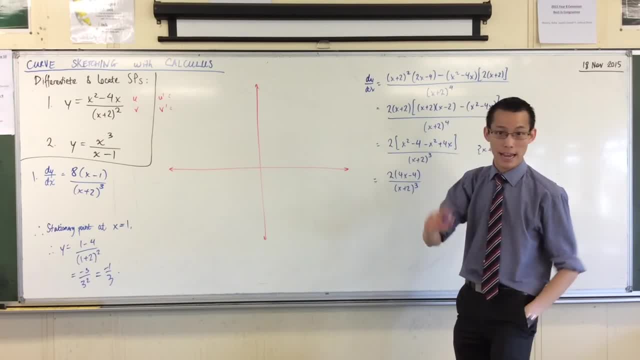 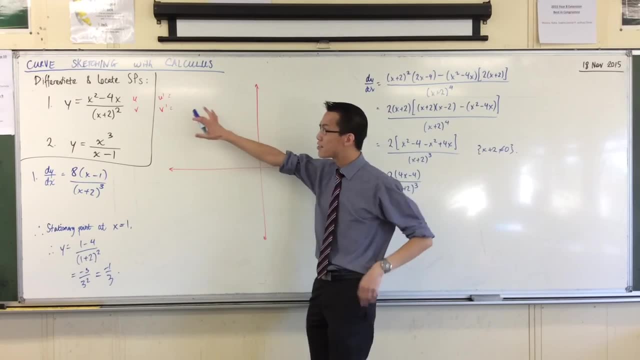 I'll know exactly where to put my stationary point, And there's only one. That's kind of handy to know. All right, now that that's out of the way, as a preliminary sort of thought, I can do this kind of thing with all of the non-calculus tools I've already taught you.